And how does it play the hydrogeology of that all? 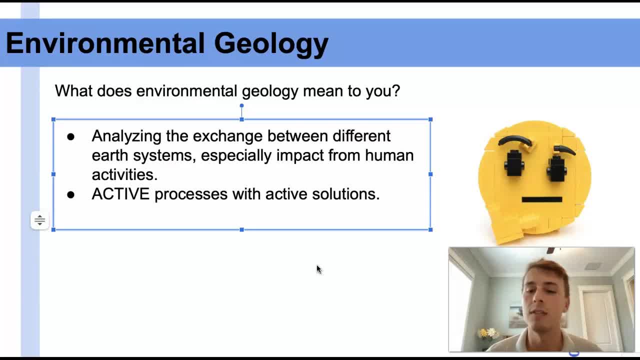 To me, compared to other geological fields of study like volcanology or seismology, these are really active processes that we're studying here. 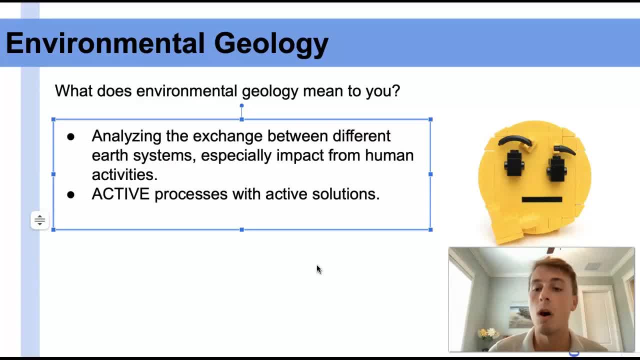 With mineralogy and different types of hard geologists, you're studying a record of something that happened millions of years ago, whereas environmental geology is focusing on the processes and things that are happening right now. 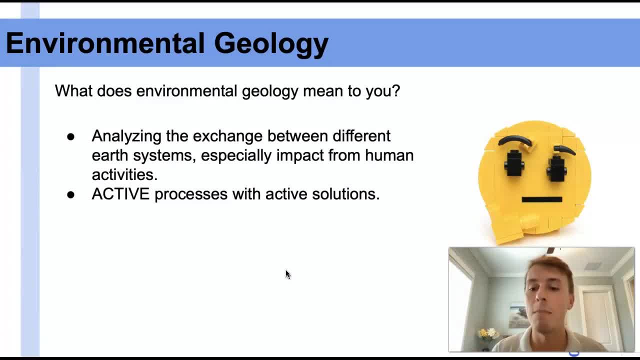 And mainly that's because they are focusing on impacts from human activities or the impacts of geology and the environment on human activities. 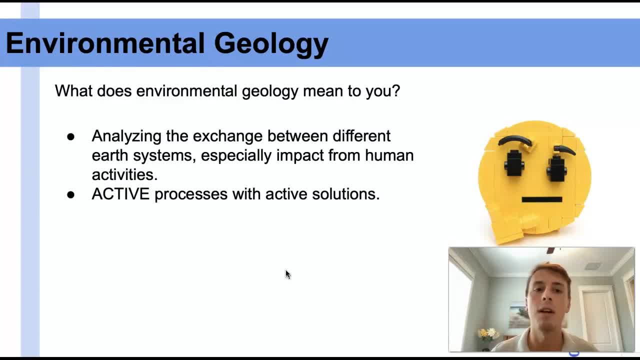 So these are active processes, which I find a bit more interesting and often have active solutions. 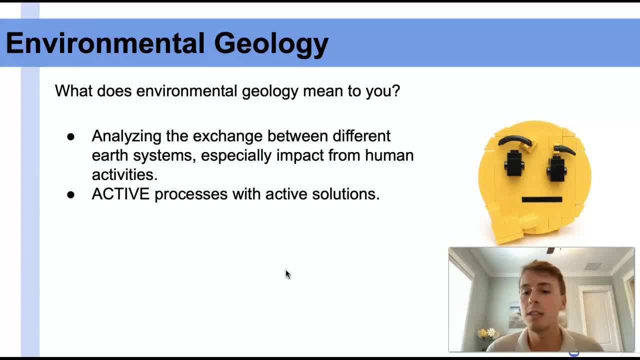 These are things that are currently happening and there are solutions to them. That's when you start moving into the field of engineering. 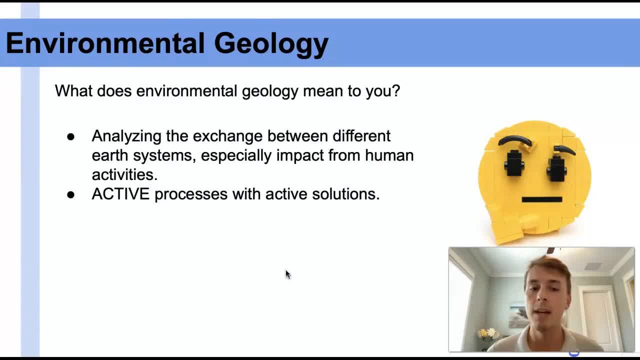 Where you're designing and implementing things. But these things that you study potentially can be resolved and prevented from happening for future generations. 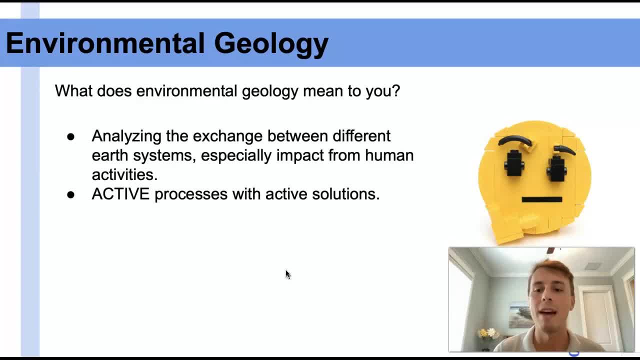 And so I find that quite fulfilling to have that feedback and interplay with every real life application. 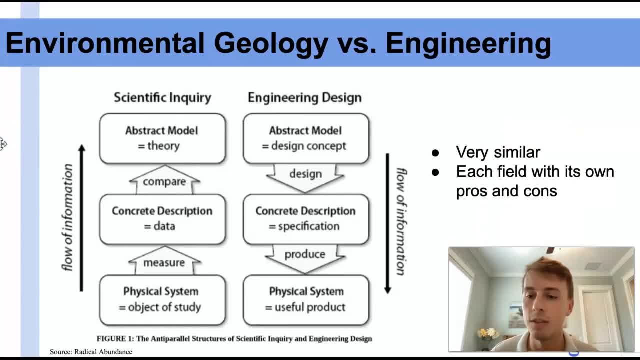 So comparing environmental geology to environmental engineering, which I am an environmental engineer. And it really gets down to the differences between science and engineering, because there are differences to your approach to a problem. 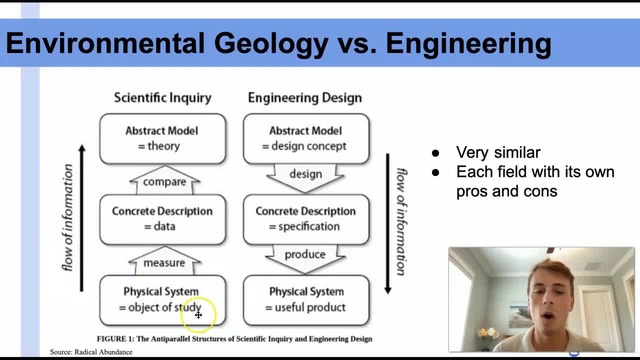 So a scientific inquiry starts with something that already exists, a physical system that's already present. 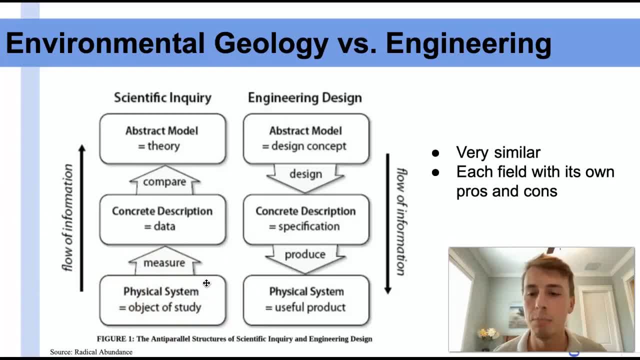 There is some scientific anomaly that we can't explain. And so we take measurements, we try to describe it, and eventually turn that into an abstract model. That can then turn into an abstract model. 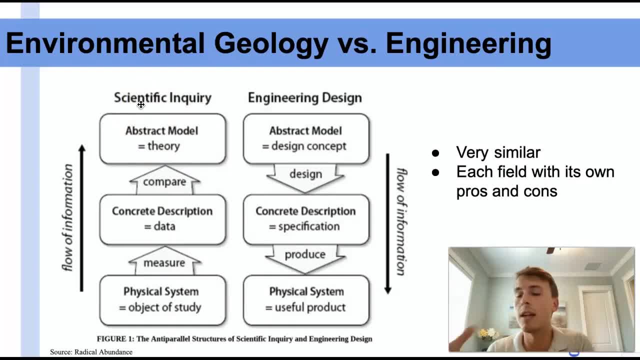 That can then turn in term guide our expectation of how that system will behave in the future. 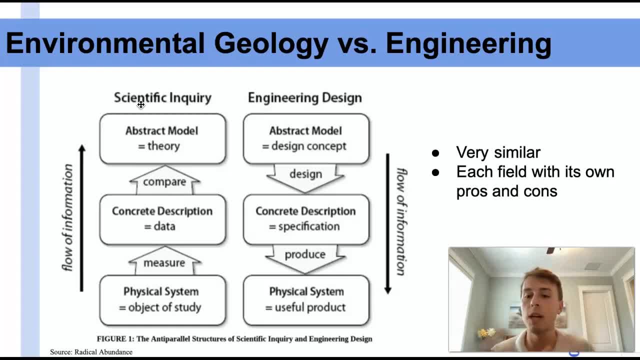 So we're studying something, we're trying to develop a generalization that we can make about it. That we can apply to a system like that in the future. 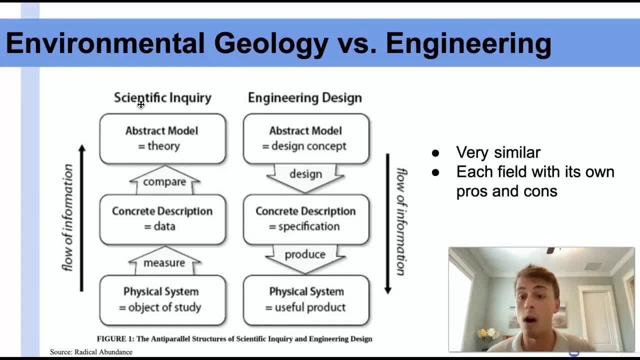 Whereas engineering design takes these abstract models that are often developed by scientists, the way we expect things to happen has been developed by a scientist. And so an engineer can take a model and say, hey, I know what you're talking about. An engineer can take that expectation, take that model, design something that then turns into a physical system. So I know water flows this way, and so I'm able to make a water treatment plant that flows in the same way and uses these equations and flows that have been determined by scientific inquiry. 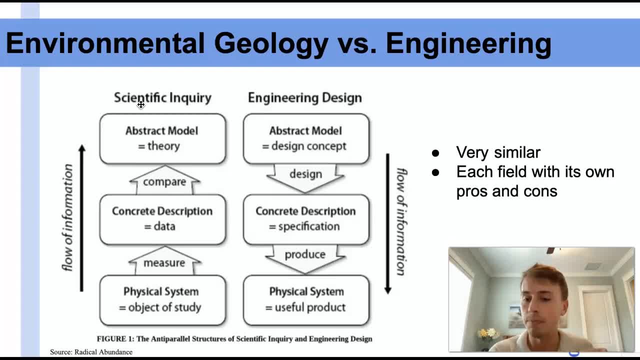 So there's really a fundamental exploratory inquiry that's happening with science, and engineering is application of that in real life. 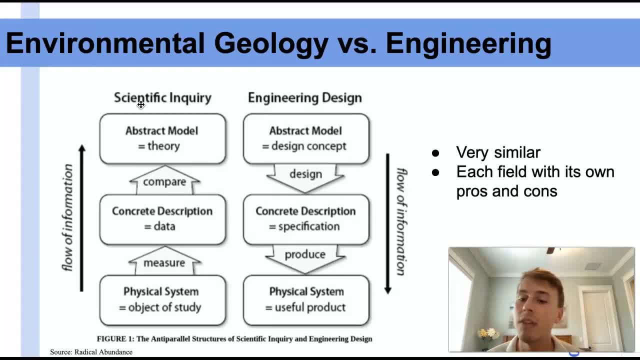 So these are very similar fields, but each have their own pros and cons. Science just tends to take a lot longer. 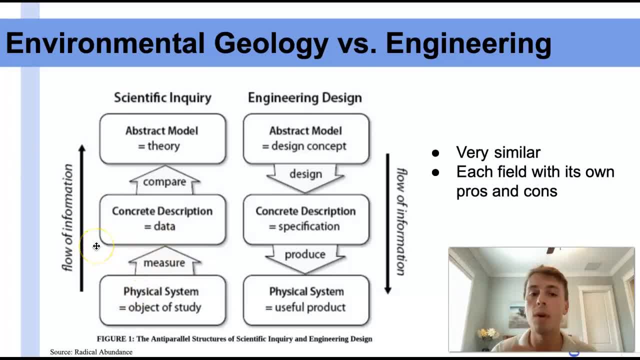 You're taking a lot of measurements off often before you can interpolate that and turn that into a model. 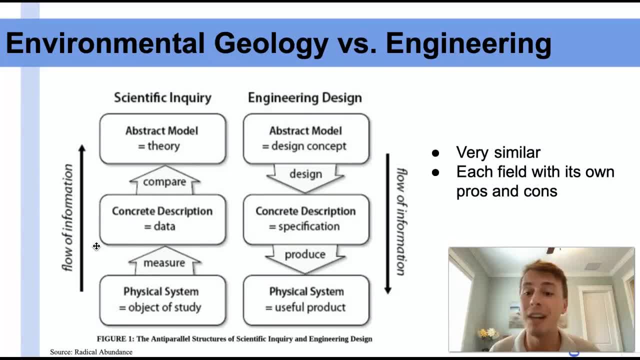 Engineering, on the other hand, happens very quickly. 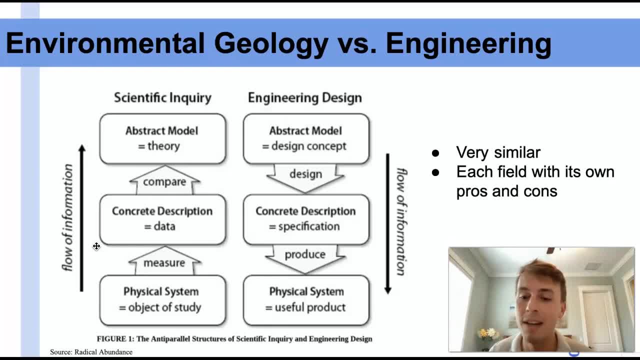 You tend to expect the way things happen, and sometimes that's not always correct. Your assumptions don't end up being true, but you're able to take concepts and hopefully 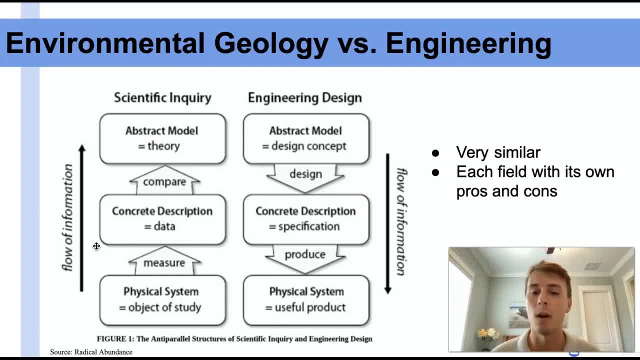 cross your fingers, turn it into something that actually works. 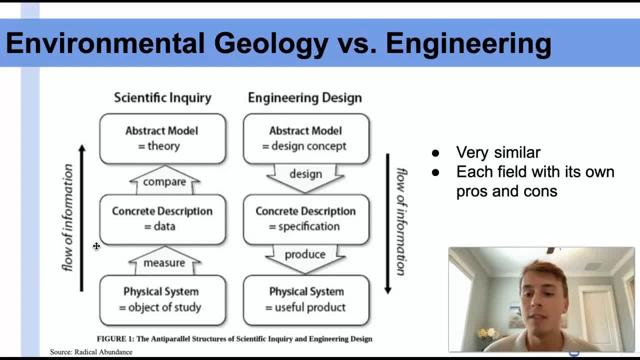 So scientific inquiry moves a lot slower. It definitely is more thorough than engineering processes tend to be. Whereas engineering design is about rapid implementation in the field often. And that concludes our lecture. 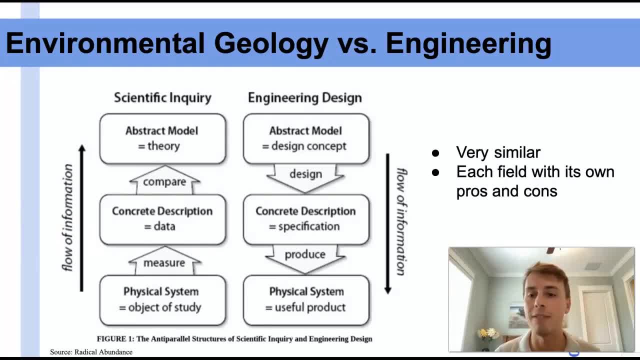 Please don't hesitate to reach out with any questions you may have.